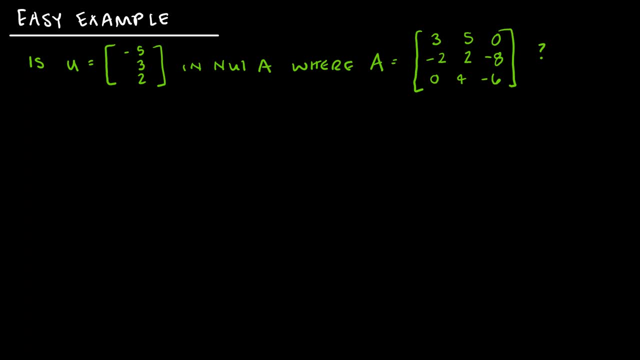 just requires computation. So the question says: is u in null a? and they give us a which is a three by three matrix. So what we know about null is that null a is the set, I whole set- of all x's, such that x belongs to Rn and ax equals zero. 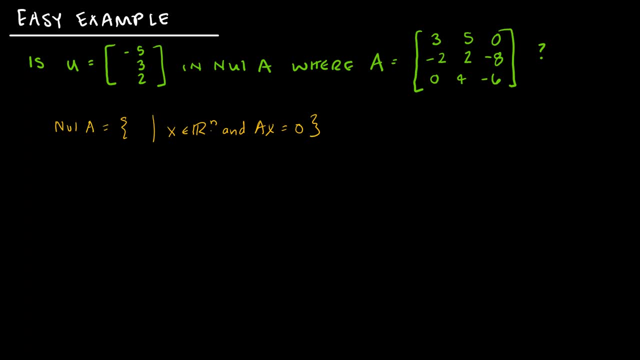 So essentially in this case, I'm saying: is u one of those values? So is u a solution to this? So that's pretty easy to check. I can take a times a u and find out what that is, And if it's equal to 0, then u is in null. So let's take a look. 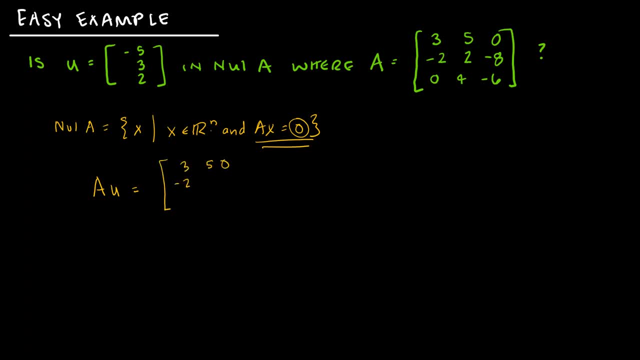 a times u would be 3, 5, 0, negative 2, 2, negative 8, 0, 4, negative 6, multiplying by u negative 5, 3, 2.. Let's do our matrix multiplication So I would get negative 15 plus 15 plus 0. 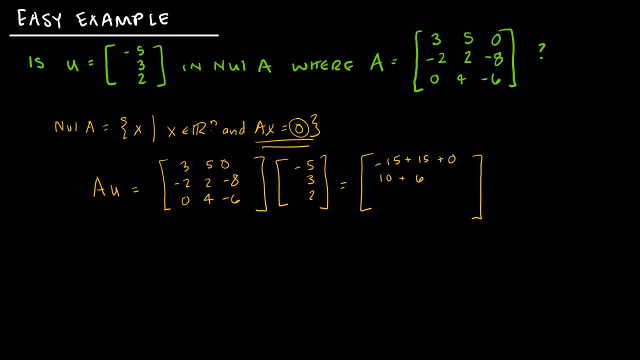 I would get 10 plus 6 plus negative 16, and I would get 0 plus 12 plus negative 12.. And if I take the sum, I would get 0 and 0 and 0. And because that equals 0,. 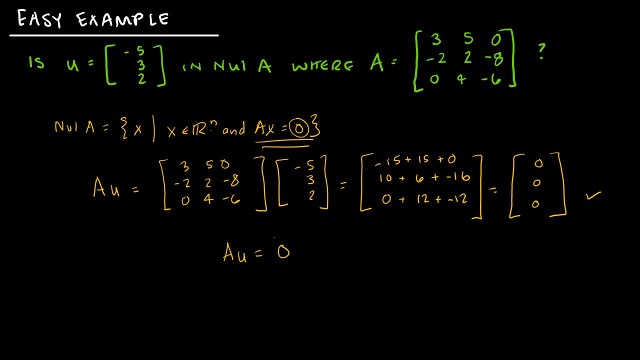 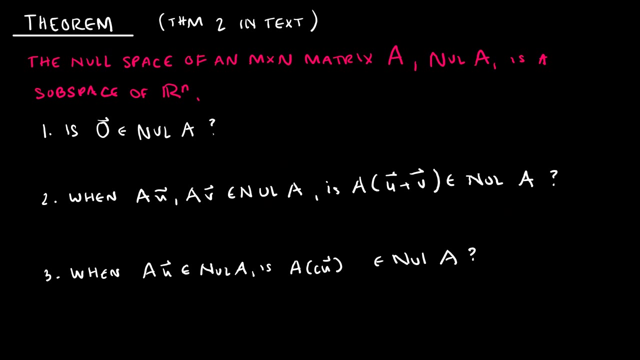 so, essentially, I've shown that au is equal to the 0 vector and therefore, yes, u is in null a. This brings us to our proof of whether or not a null space is in fact a subspace. So recall a couple of definitions. First of all, we have to recall that when I'm talking about null, 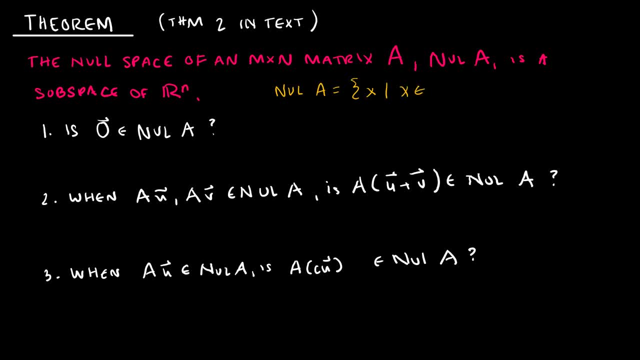 a- I'm talking about all of the x's, such that x is an element of Rn and ax equals 0. That's our definition. I also need to remember the definition of a subspace, And the subspace has three properties. First, that the 0 vector belongs to the subspace, that it is closed under addition and it is closed under scalar multiplication. 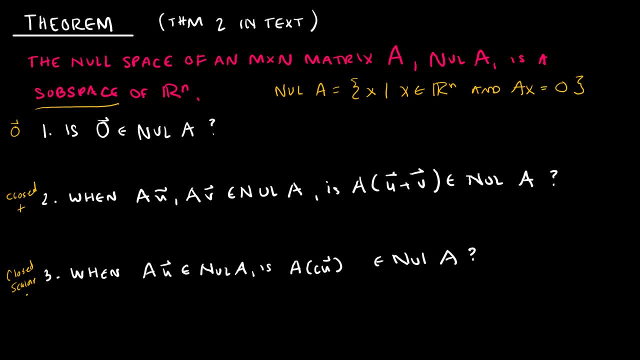 So that's the three that I have written here, but I have them written out in a way to help me to know exactly how am I going to check that condition? So first of all, is the 0 vector in null? So what I know is that null a is the set of all x's, such that ax equals 0.. 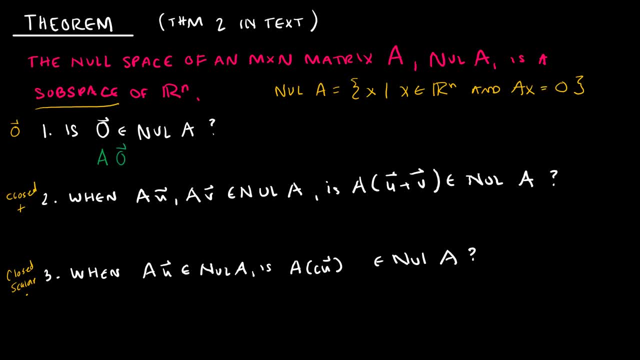 So essentially I'm asking: is a times 0, does that equal the 0 vector? And, of course, a times 0,, or anything times the 0 vector is going to equal the 0 vector. So yes, this is in fact true. 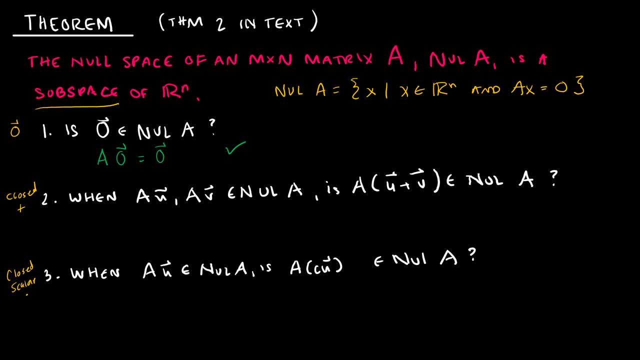 a times the 0 vector is a 0 vector and therefore 0.. I guess I should have written that. Therefore, 0 belongs to null a What else? Well, I'll have to check if it's closed under addition. 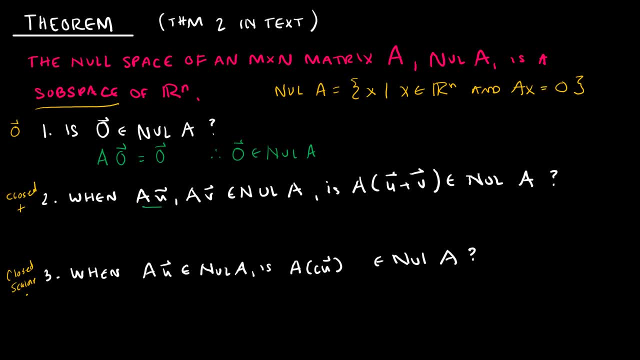 So we already know that au and av are in null a, which tells me au is equal to 0, and av is equal to 0. The question is: is au plus v equal to null a, Or is this also equal? So let's take a look. 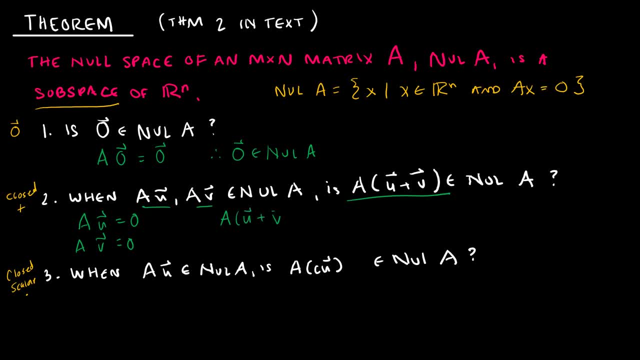 We have au plus v and I've got some properties that I've already learned about. that says, hey, if I've got something like this, I can rewrite and split them up. So au plus v is the same as au plus av. 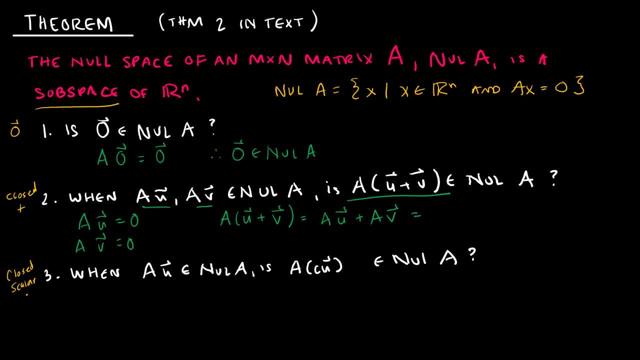 That's just the distributive property. Well, au is 0, and av is the 0 vector And 0 vector. 0 vector Plus the 0 vector is the 0 vector. Therefore, au plus v belongs to null a. 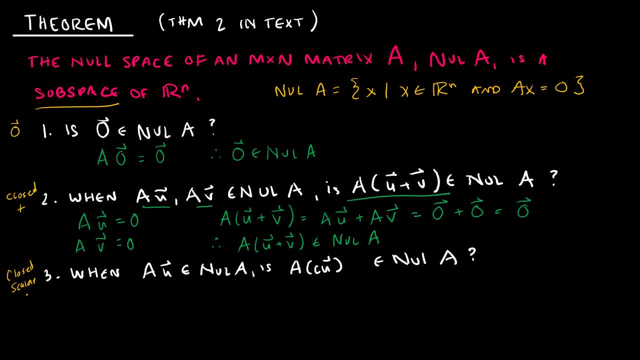 So two down, one to go. The last one is: is it closed under scalar multiplication? So when au belongs to null a- and again that's code for au equals 0, is acu also in null a? I think I said equal. 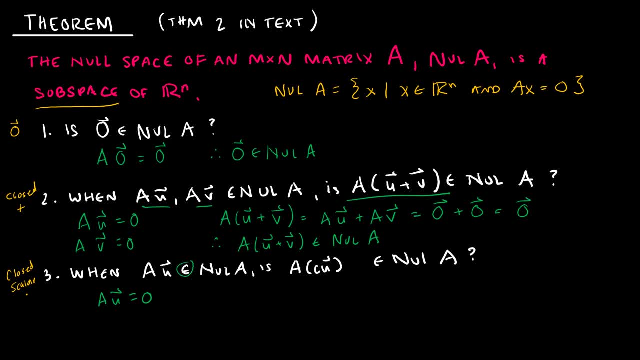 I think I said equals before. That's not: equals Is a set in. So let's take a look and see I've got a oops. sorry about that, cu, And again I can use my properties And my properties tell me that I can rewrite this as cau. 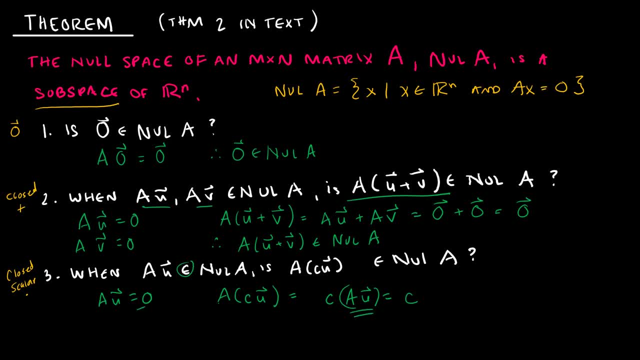 And cau means au, And I can do that. if I say that i, I can write one of my properties, So u squared is equal to 0. So c times 0. And that, of course, is 0. Therefore, acu does belong, oops does belong- in null a. 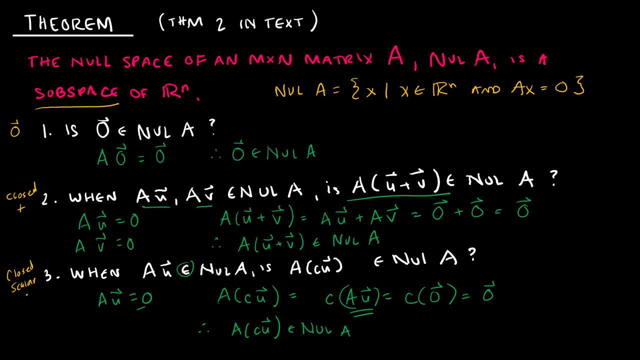 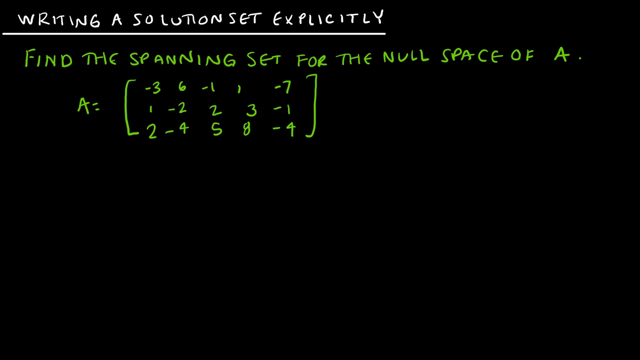 So I've proven all three of them. Therefore, what am I saying? That null a is a subspace of Rn. Done and done. What we've done so far is we have just checked to see whether a specific vector was part of the null space of A. What I want to do now is actually write our solution. 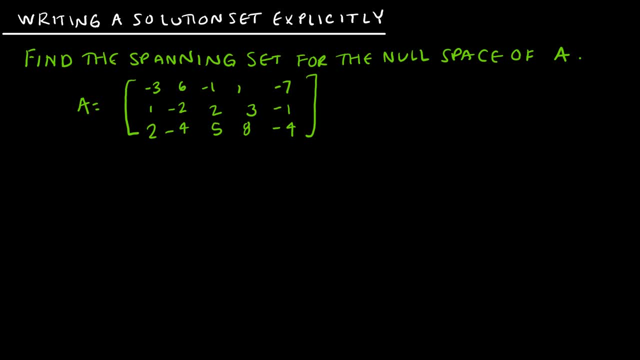 set explicitly, which means essentially we're looking at finding that general solution. We're looking at the spanning set. so I'm looking for what vectors will span the null space of A. So what I'm doing here is essentially: I have an augmented matrix and I am going to 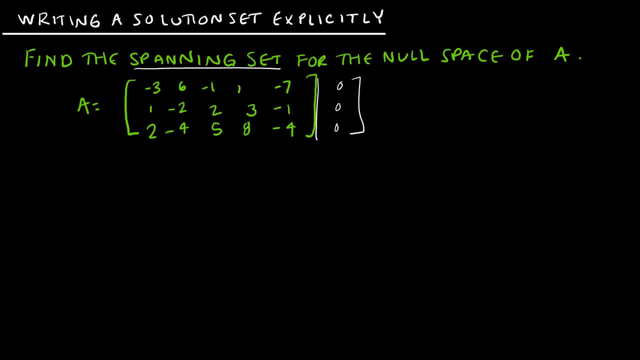 get this down to reduced row echelon form and then I'm going to write my solution parametrically. So let's all things that we know how to do so far, but let's go ahead and work through this one together. So I'm going to take three times row two plus row one to be my new. 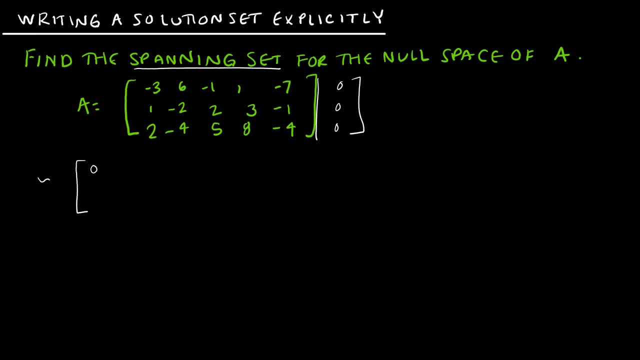 row one. So that gives me three plus negative three is zero negative. six plus six is zero. six plus negative one is five. And again I'm going to end up switching these rows, which is why I'm making that a zero. Let's see what was I doing. I was taking three times row. 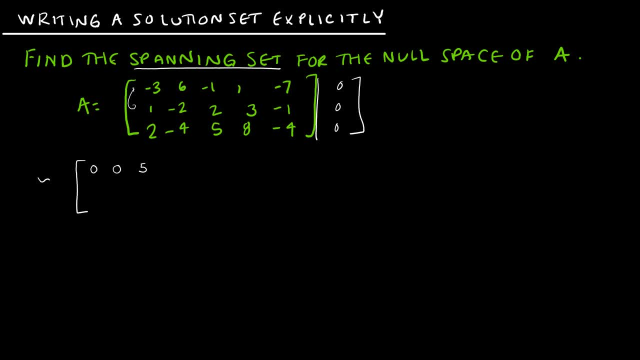 two, so that's six plus negative one is five. nine plus one is ten. negative. three plus negative seven is negative ten. and this row I'm going to keep just as it is, because I'm going to flip-flop those, because I want that one in my very first entry. But let's. 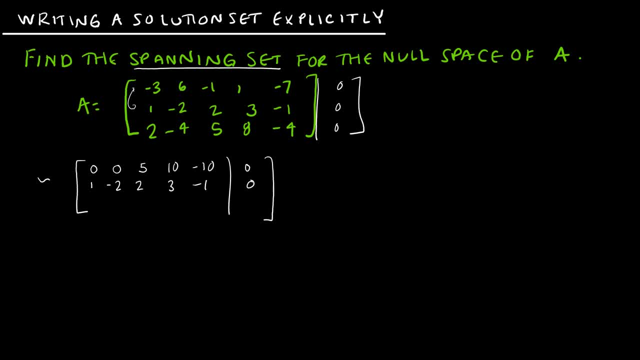 go ahead and make that last one a zero as well. So negative one, I'm sorry, negative two times row two plus row three. So negative two plus two is zero. Positive four plus negative four is zero. Negative. four plus five is one. 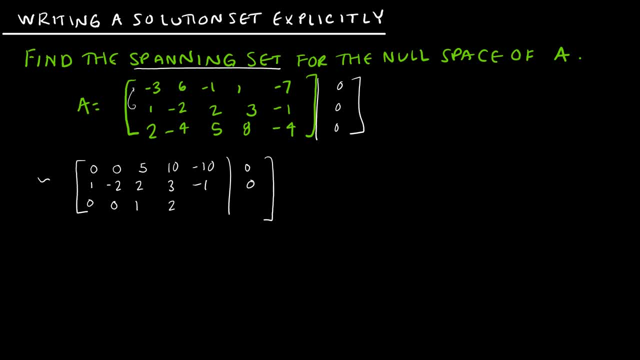 Negative six plus eight is two. Positive two plus negative four is negative two. I'm going to put this as my first row and I'm just going to recopy: Zero, zero five, ten negative three. zero five, ten, zero and zero, zero one, two negative two. 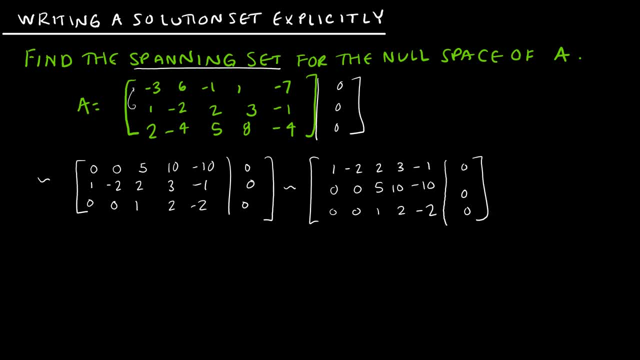 And now what? Well, now I can see that I can let me just put it down here My second. no, you know what? I'm going to put it up here because I need to make sure I have enough room. I'm noticing the relationship between these values, and so what I'm going to do is I'm 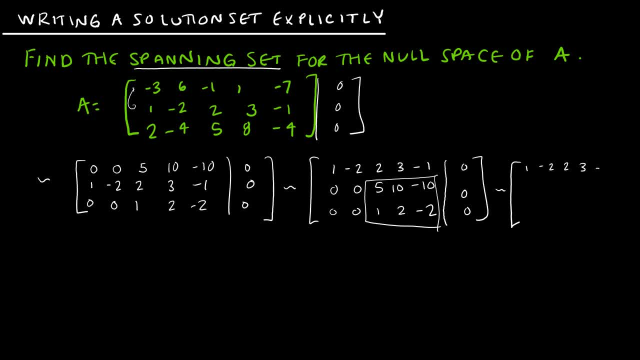 going to leave this first guy the same. Oh, I got a little overzealous with that. one Negative, one zero, And then my middle row. I'm going to take it times one-fifth. So that's one. two negative two. 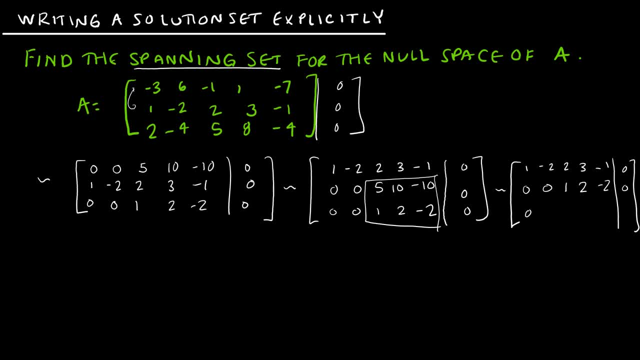 And then I can see that I can very easily make these all zeros because they're the same. And so just by you know, combining um taking row three times negative five, or taking a fifth of row two and adding it to row. 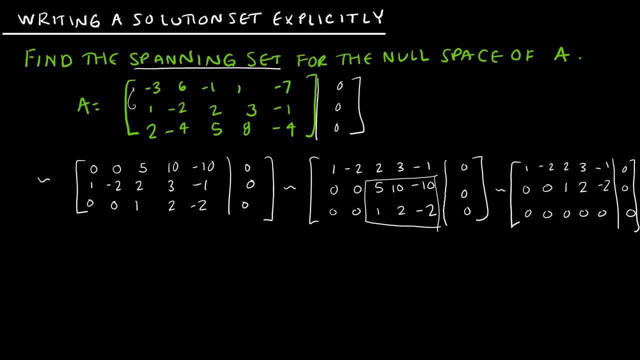 three. you get the idea. So here's where I am, and this is really good, because obviously I have my pivot here and I have my pivot here. So the only thing that's wrong now is I need that guy to also be a zero, And that's a step that a lot of us are missing. as I'm looking at people's work, 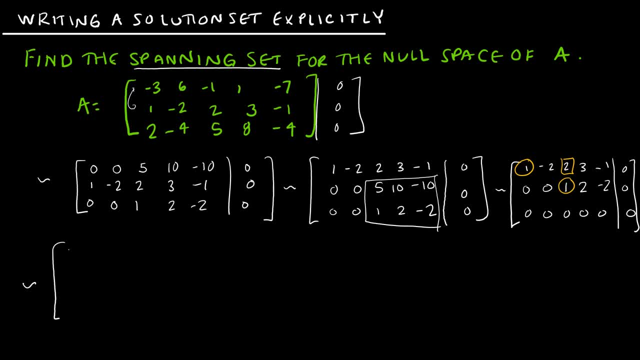 is. we're missing that step, So don't forget that step. Just because you have your pivots does not mean you're done. So my first row. I'm going to take negative two times my second row and add it to my first row. So these first two terms aren't going to change because I'm adding. 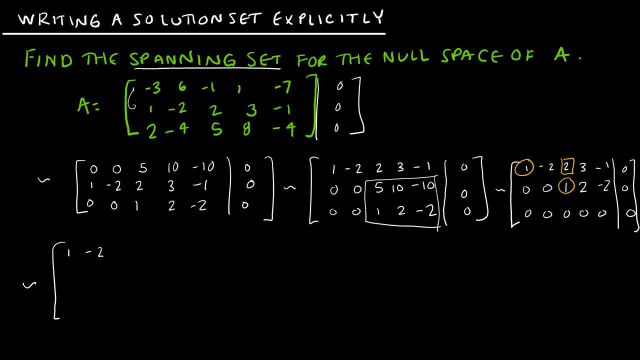 negative two times zero. So negative two times one is negative. two plus two is zero. Negative two times two is negative. four plus three is negative one And negative two times negative. two is positive. four plus negative one is three. And then my second row. 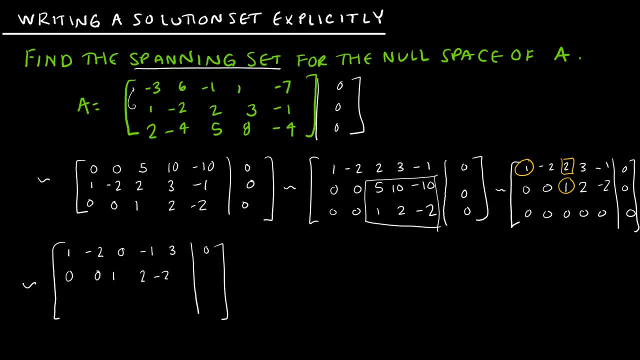 is fine. My third row: all zeros. And so again, what do I want to do here? I want to write this in, basically using what my free variables are. So here's my pivot and here's my pivot, which means: x2 is free, x4 is free, x5 is free. 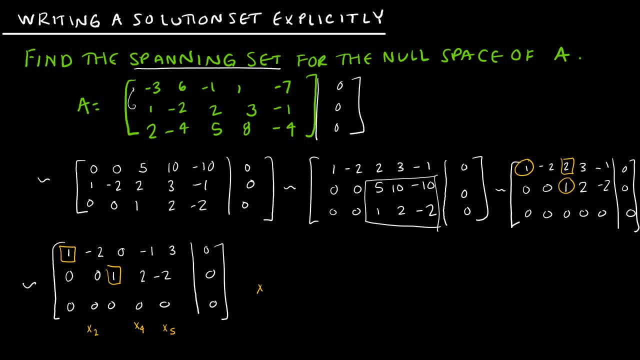 So those are my free variables And that's what my solution is going to look like is using these guys as my free variables. So, for instance, x1 is equal to positive 2x2 plus 1x4 minus 3x5.. I couldn't show you that step in between, I apologize. 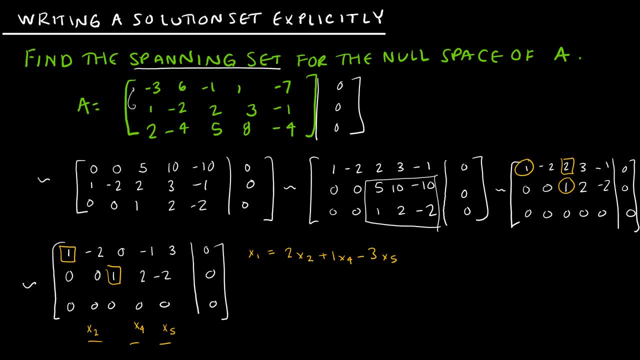 but hopefully we've done this enough that we understand how to do it. x3 can be written in terms of our free variables. So x3 is negative 2x4, positive 2x5.. And that's it. So how am I going to write this solution? I am going to write it as: 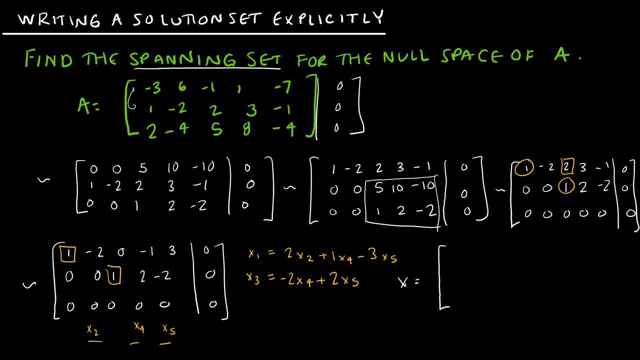 there we go. x equals, And then my first free variable is x2.. And what do I have for x2?? I have 2 for x1.. For x2, that's free, so it's a 1. For x3,. 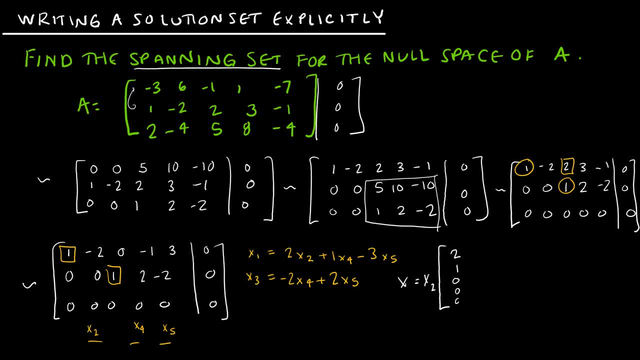 I've got negative. nope, I've got nothing. And I've got nothing for x4 or x5.. And then, plus, my next free variable is x4.. And x4 is, there's one of them in x1.. 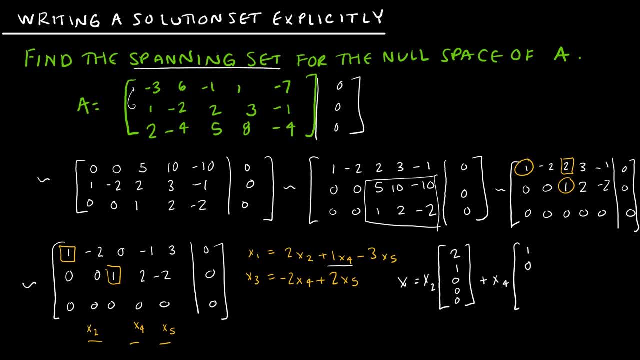 There's negative 2 of them in x3. So there's none of them in x2.. Negative 2 in x3.. x4 itself is free, so don't forget the 1.. And then none in x5. And then x5. And then for. 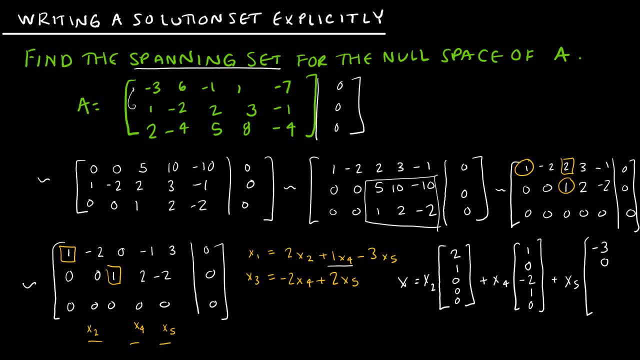 x1, it's negative, 3x5s. Nothing for x2, which is free. x3 is 2x5.. So that's 2x5.. x4, nothing because it's free. x5 is free, so don't forget the 1.. 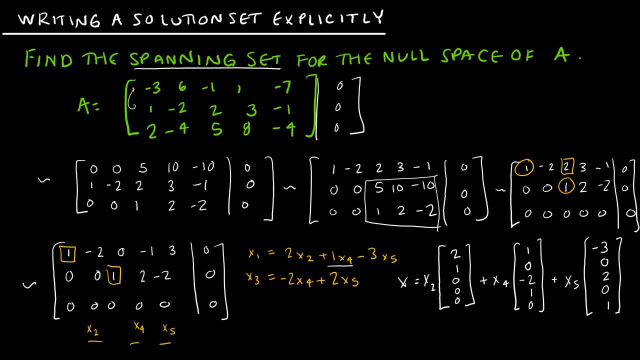 So am I done? Did I answer the question? The question says: find the spanning set for the null space of a, And again that means x can be written. if this is u and v and w, then any solution here? 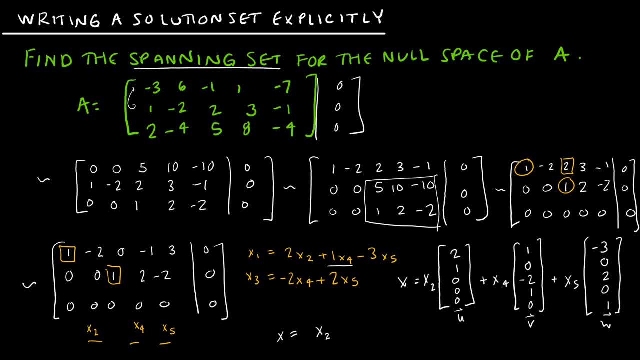 can be written as X2U plus X4V plus X5W. So I have answered the. I've basically simplified the question. The spanning set is all of the vectors 2, 1, 0, 0, 0. 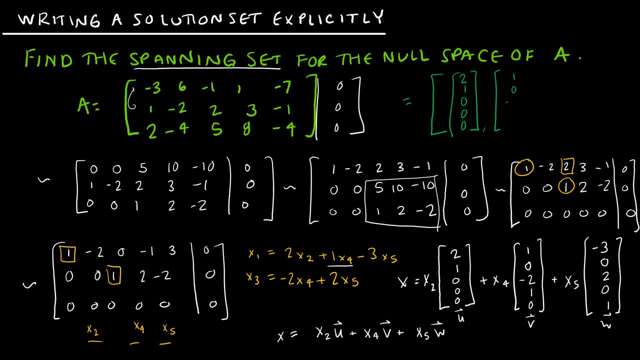 It's the set of all of those vectors, So 1, 0, negative 2, 1, 0, and negative 3, 0, 2, 0, 1.. So that is the spanning set. is that those set of vectors, the vectors U, V and W? 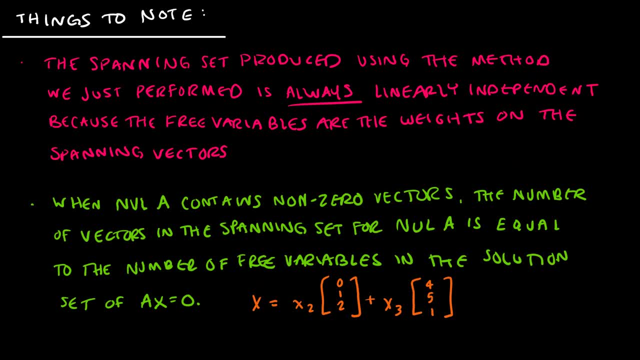 So just two things to keep in mind regarding what we just did. Keep in mind that the spanning set, produced using the method that we just performed, is always linearly independent, because the free variables are the same. They're the weights on the spanning variables. 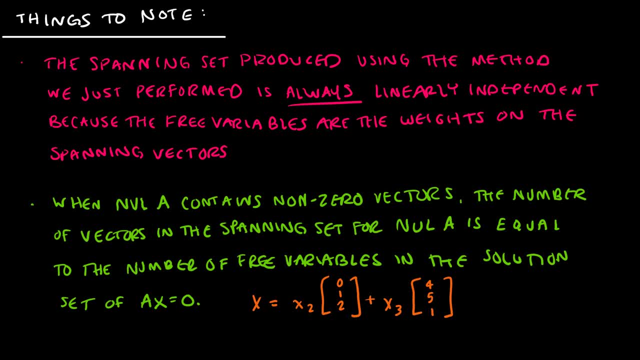 So, going through that process, we know that those three vectors that I just came up with are linearly independent, Again, because we have the free variables times the weights of the spanning vectors, And when null A contains non-zero vectors, then the number of vectors in the spanning set for null A is equal to the number of free variables. 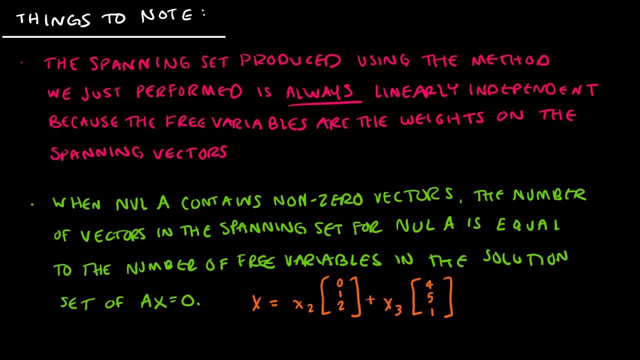 in the solution set of AX equals 0. So for instance, say: this is my, this is my solution. Notice: this is a free variable, This is a free variable. So the number of vectors in the spanning set is equal to the number of free variables. 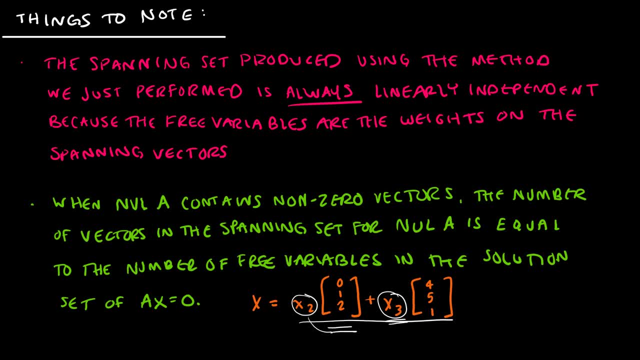 So notice: one free variable times one vector, one free variable times one vector. So it makes sense that those would match up. The number of free variables would match up with the number of vectors.